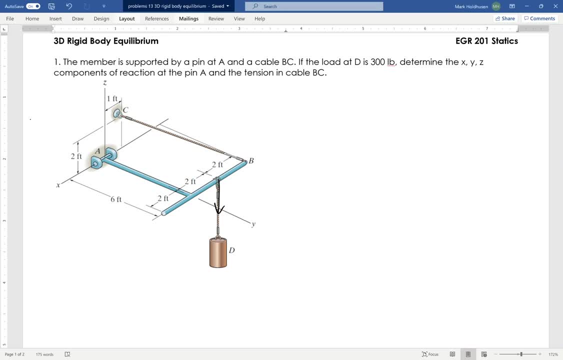 Okay, I've got a member here that's got a pin at A and a cable B, C and it's loaded up with 300 pound weight, as shown at D. Okay, and I want to find the X, Y, Z components of pin A and figure out that tension in the cable. So we'll start with the free body diagram which I'll draw right on top of the body here. So again, I've got 300 pounds acting straight down. That's in pounds, so I don't need to convert it with gravity or anything. 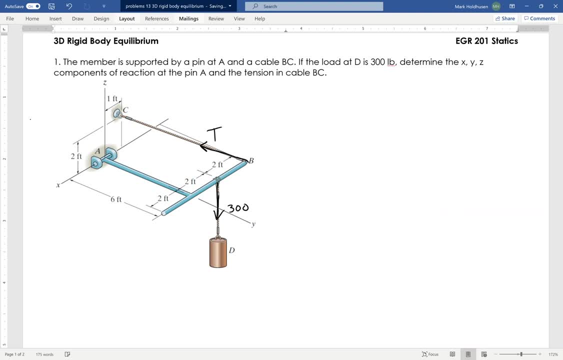 It's already given as a force. I've got my tension over here at B, which we'll go through and write the Cartesian form of in a second, And then I've got some stuff going on at A. So again, what we're looking for is what I can't do, And because of the pin I can't move in the X direction, cannot move in the Y direction and I cannot move in the Z direction either. Okay, so that means I've got an AX, an AY and an AZ. 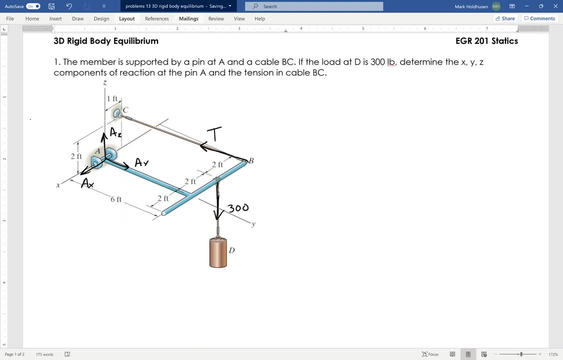 So I've got an A component at that pin joint, because I can't move linearly in any direction. Now what I can do is I can rotate about the X axis. Okay, so there is no reaction about the X axis, no reaction moment. 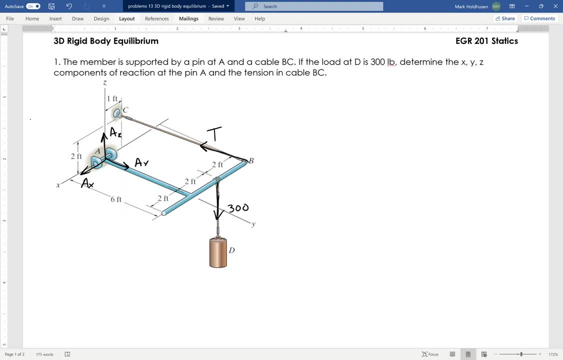 However, if I try to twist that or rotate it about the Y or the Z axis, that pin joint restricts that motion. So there would be a reaction moment about the Z axis. However, if I try to twist that or rotate it about the Z axis, that pin joint restricts that motion. So there would be a reaction moment about the X axis as well as about the Y axis. 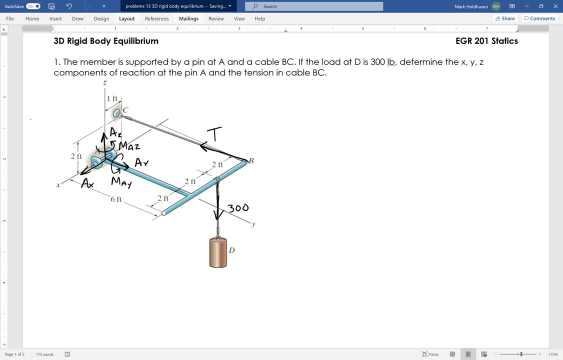 So we'll go ahead and draw in there the moment about the Z, moment about the Y, Again, not one about the X axis, because it's free to move, It's free to rotate around that axis. So there's no reaction moment there. 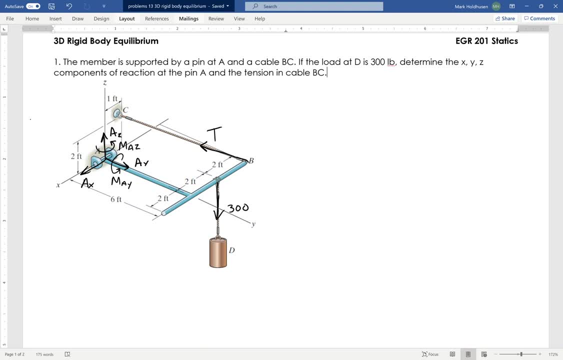 So before I go ahead and get into my equilibrium equations, the first thing I'm going to do is go ahead and draw my- not draw write my- tension in Cartesian form. So that's an unknown tension. but I need the unit vector, so that's the position vector over its magnitude. So, going from B to C, I go 3 in the I direction. 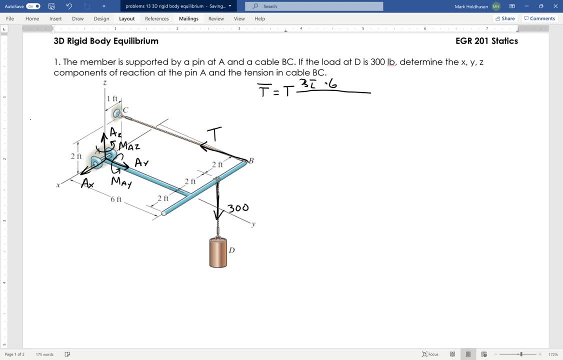 I go 9 minus 6 in the J direction and then I go up 2 in the K direction. Now we've seen this before. It's a 2,, 3, 6, 7 sort of situation here. 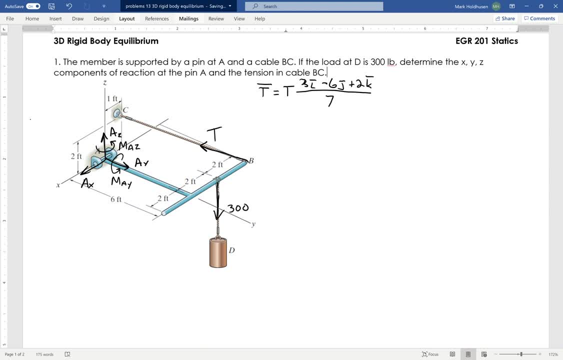 So the magnitude: square root of the sum of the squares. So that gives me that. So now that I've got this, I'm going to go ahead and deal with my reaction forces. I'm sorry, not my reaction forces. I'm going to sum my forces in the X direction. 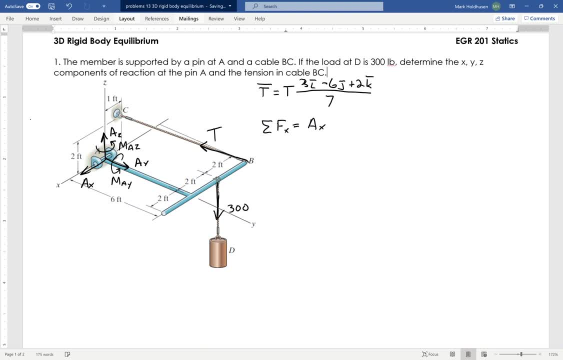 So I've got my reaction AX there and then I've got this tension right which is 3, 7ths times the tension in the X direction. That's all I've got going on in the X direction. so I set that equal to 0.. 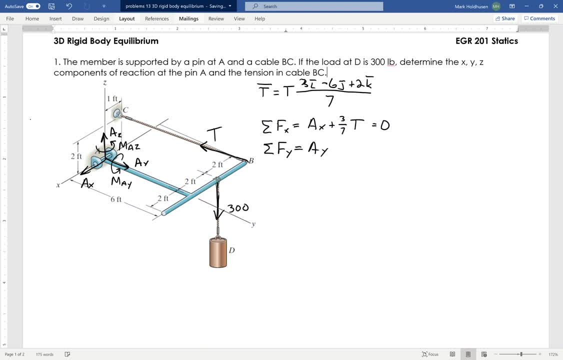 Similarly in the Y direction, I've got AY And I've got minus 6 7ths times T and that's all I've got in the Y direction. Now in the Z direction, I have the AZ, I also have the 2 7ths T, but I also have the 300 acting straight down. That's that weight that I've got applied there, so I'm going to go ahead and include that. 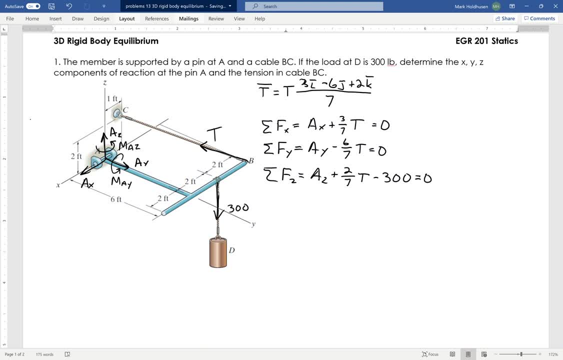 Now, these are three equations, right, but I've got four unknowns: AX, AY, AZ and T, so I'm going to need more equations. Fortunately, I have moment equations. Unfortunately, those moment equations are in three dimensions, which makes life a little challenging. 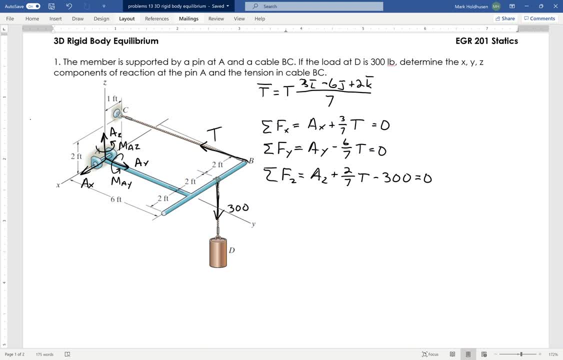 So what I'm going to do is I'm going to do some cross products and then pull out the X, Y and Z components of that moment equation. So I'm going to do this moment about point A, because AX, AY, AZ will then disappear, right? 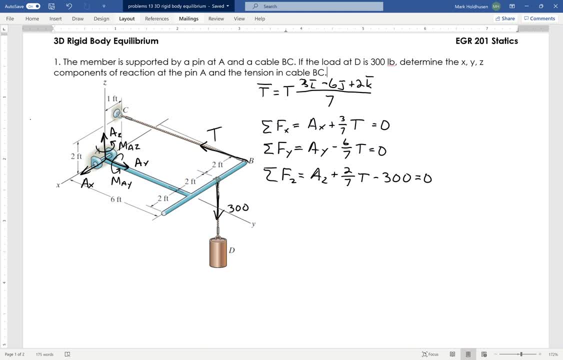 They do not create any moment about point A because they're at point A. We usually choose a point with the most unknowns at it, which obviously is point A here, So I do that. I want to include any couple moments. I get these, so don't do that okay. 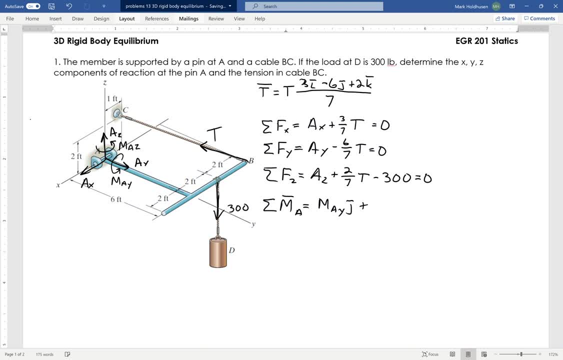 I've got my reaction moment AY and reaction moment at A about the Z axis, So you want to make sure you include those. Those are the two couple moments that I've got Now. I've got a couple of R cross Fs that I'm going to deal with, right. 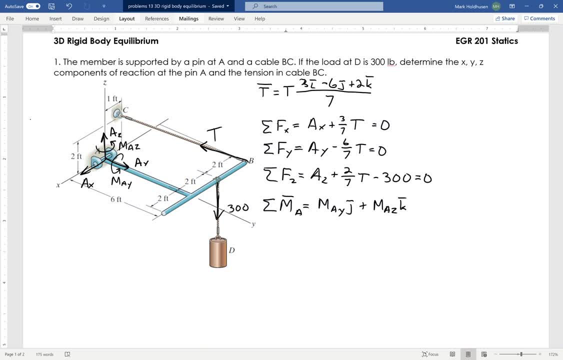 So we'll start with the 300, right. So, to go from A to that D force, I move negative 2 in the X And I move 6 in the Y And I'm going to take that and I'm going to cross it with the negative 300 in the K direction. 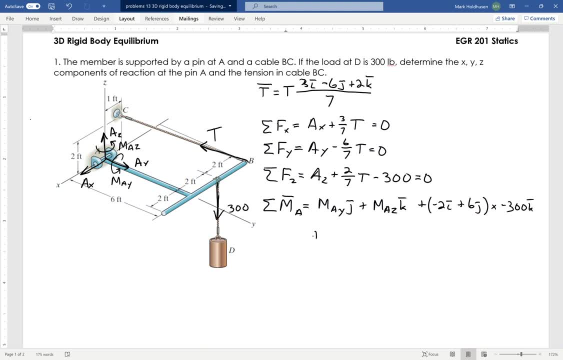 Now I'll do the same thing, going to B, okay, Where this time I'm going to go negative- 4 in the X And then 6 in the Y, like so, And then I'm going to cross that with that tension force. 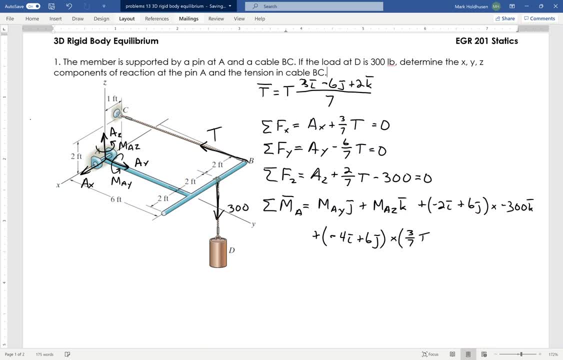 That I've got there, which again is the 3- 7ths T in the I direction, the 6 7ths T in the J direction and then the 2 7ths T in the K direction. So, doing these two cross products, I have this cross product here. 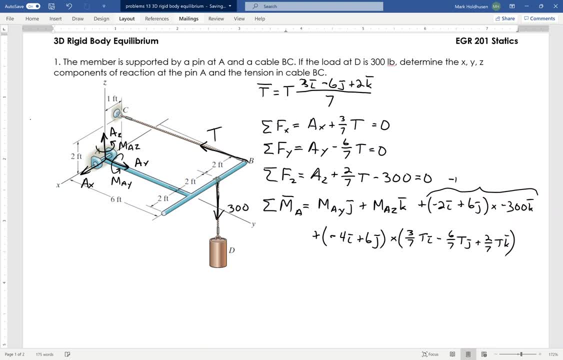 which, if I do that, I get minus 1800 I plus, I'm sorry, minus 600 J. Okay, so I'll let you do those cross products And prove that to yourself on your own. My T cross product, with the tension that I've got here, will become 12, 7ths T in the I direction. 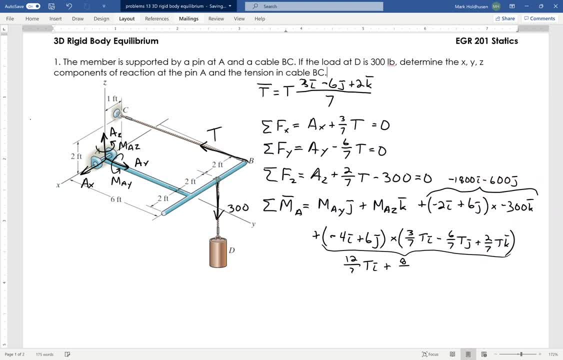 plus 8 7ths T in the J direction, plus 6 7ths T in the K direction. Okay, so now I've got all of my moments. I did. it did those cross products, kept them in three dimensions. 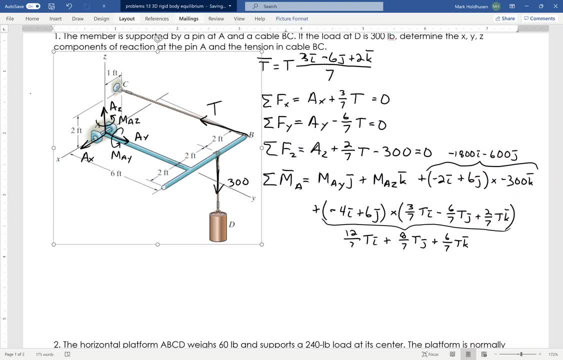 And then, um, I am now going to break them up into my X, Y and Z components. So in the X component, okay, I have minus 1800.. I've got that I component. And then I've got the plus 12 7ths T. 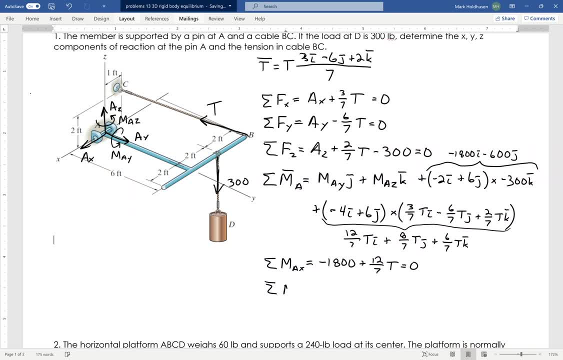 So that equals zero. Now I do the same thing with my J components. Okay, where I have M, A, Y, right the reaction moment in the Y direction, I've got minus 600. And I've got plus 8 7ths T.